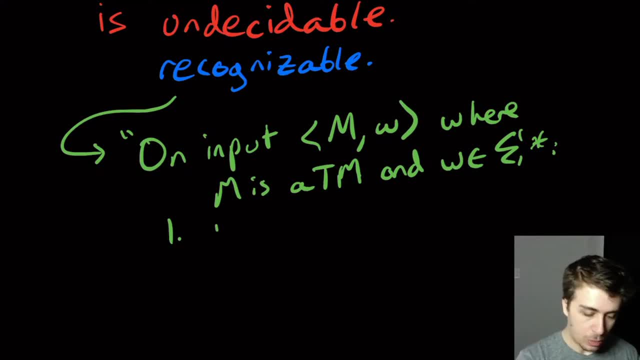 just say it's an arbitrary string And what we're going to do is just run that machine on the input W And then if it accepts, if the Turing machine M accepts W, then we are going to accept. So we will say, yes, This machine. 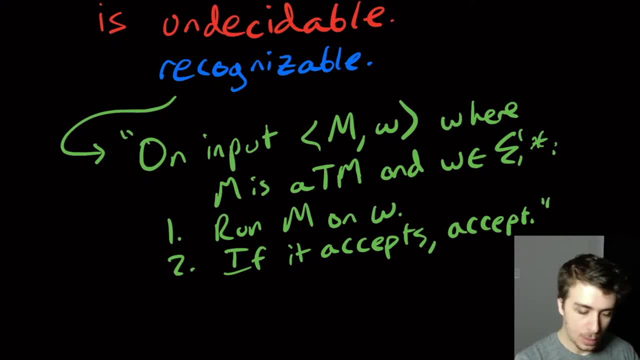 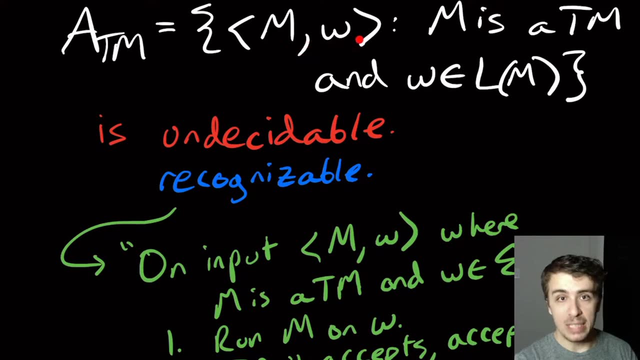 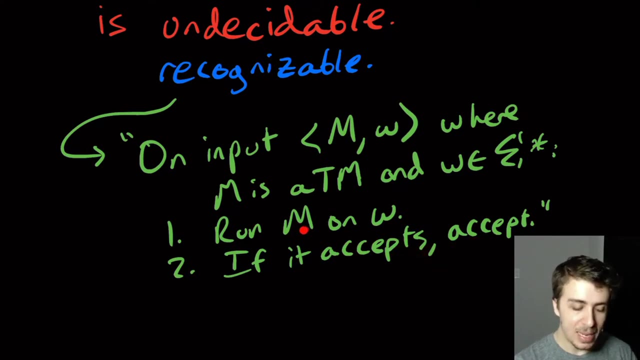 did say yes on input W, And so if the Turing machine M and W pair is really in here, that M really does accept W, well, we're going to find out that truth at some finite amount of time. But if we have, 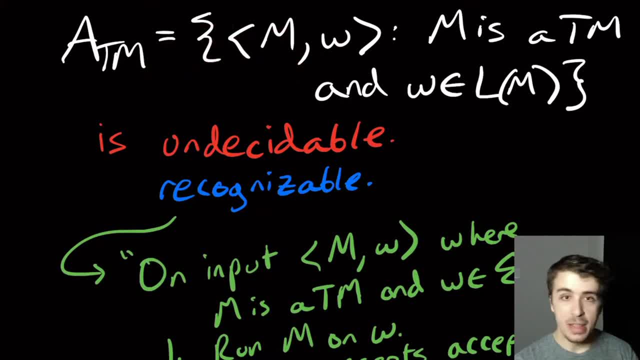 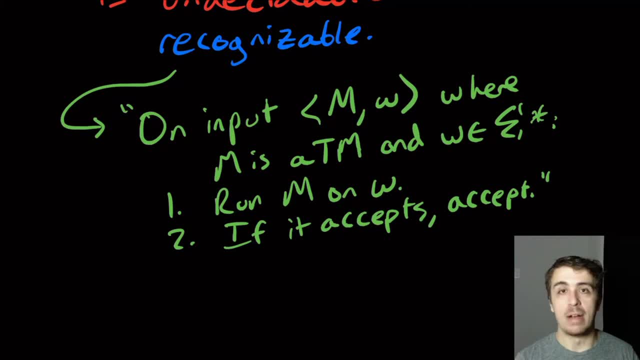 if this pair is not inside ATM here, then it does not matter what we do here. In fact, we could add a step here to say otherwise: just run forever. And if it ran forever on W anyway, we would never reach that step in the first place. So in fact we wouldn't even reach step two. 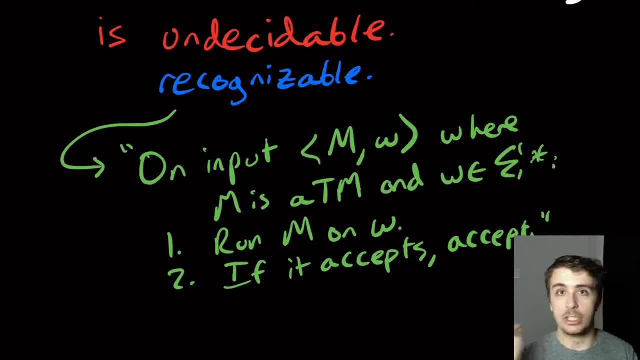 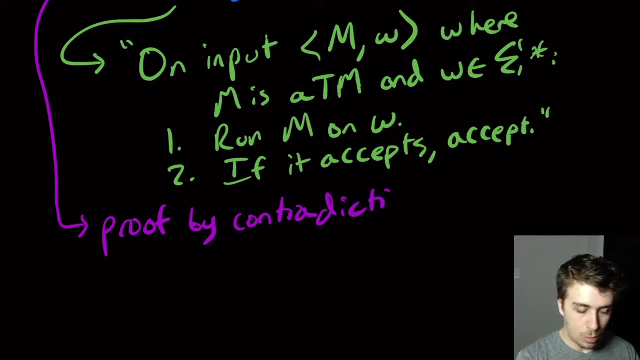 So how do I show that this is undecidable and that there is no possible algorithm for this? So the way, the common way of doing this, and it's a classic proof- is a proof by contradiction. So what we're going to assume is that there is a Turing machine for 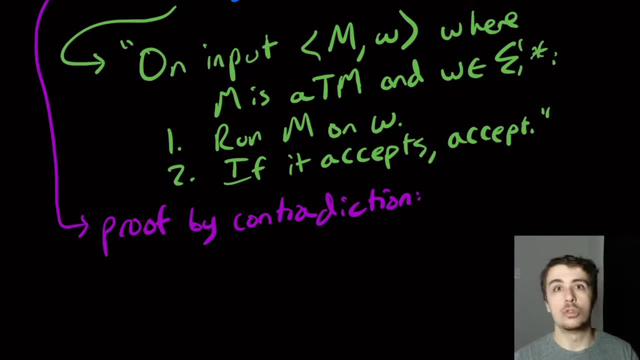 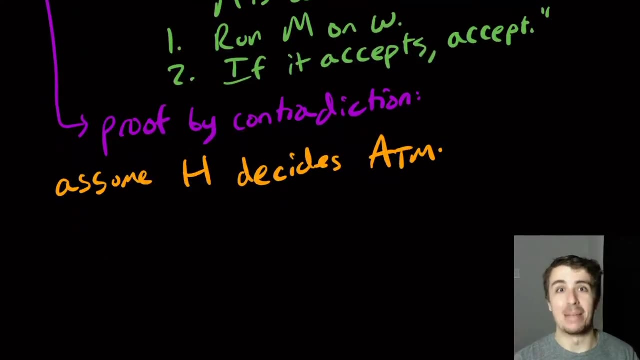 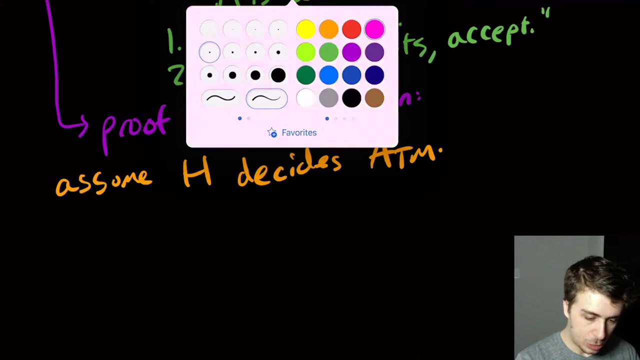 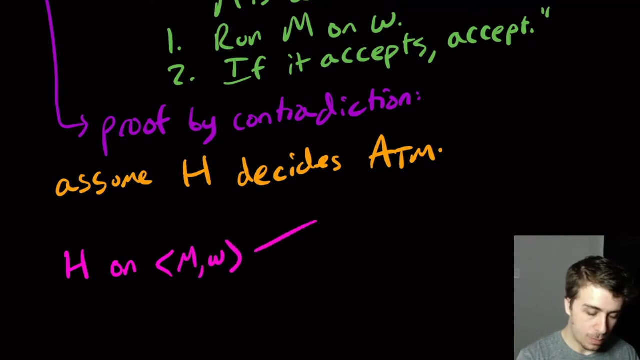 that is a decider for ATM, and then derive some kind of contradiction. So we're going to assume that H decides ATM. H stands for hypothetical. We're assuming that this machine really does decide the ATM problem, And just for posterity, H, when given the input pair M, W, since it's a decider. 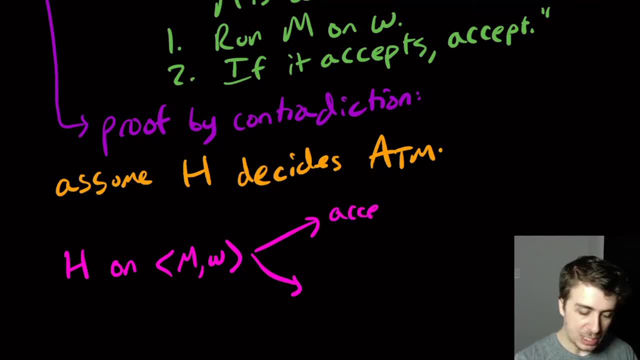 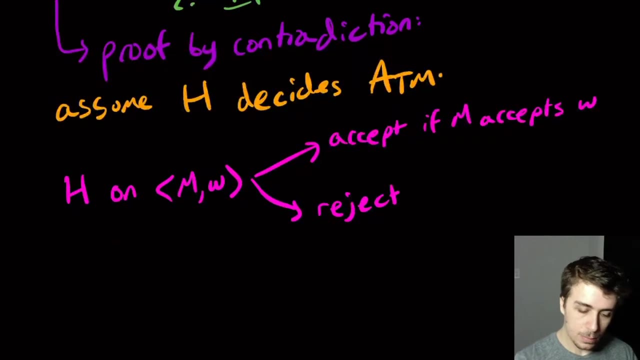 it must do one of two things: It's going to either accept or it's going to reject. It can't run forever because it's a decider by assumption. So if it says accept, that means M accepts W and it's going to reject otherwise, because that's just what the definition of the machine is. 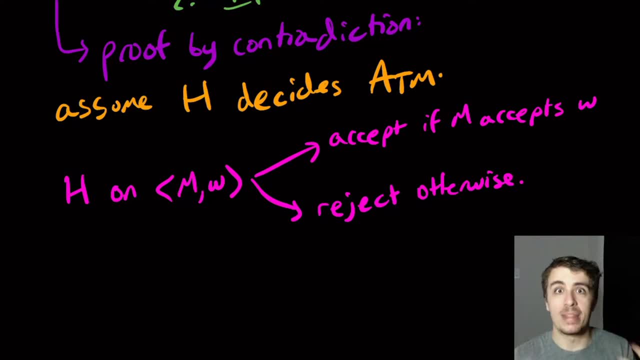 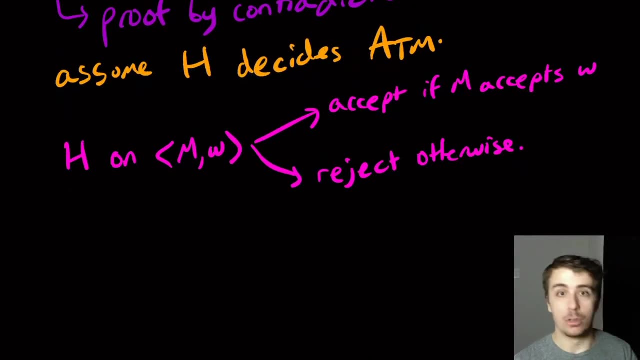 But for posterity. it's just to get a good idea of what the machine actually does, because we're going to do it on the later machine. here, In fact, the contradiction is going to come from creating another machine that will help us get a contradiction. 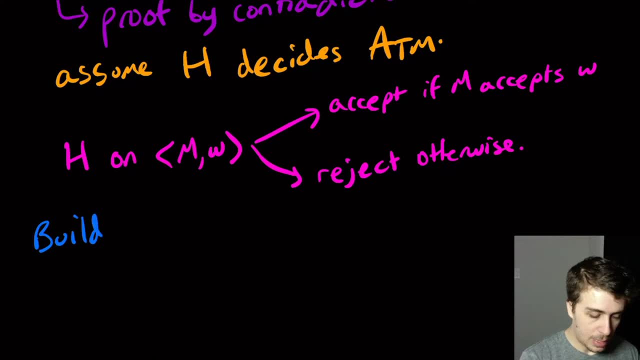 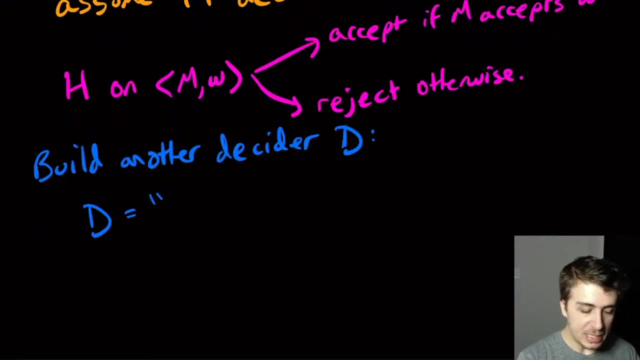 So we're going to build another decider, And for a completely different problem, but it's a decider And what it's going to do is going to do this. So D's instructions are: it's going to be given a single Turing machine and nothing else. 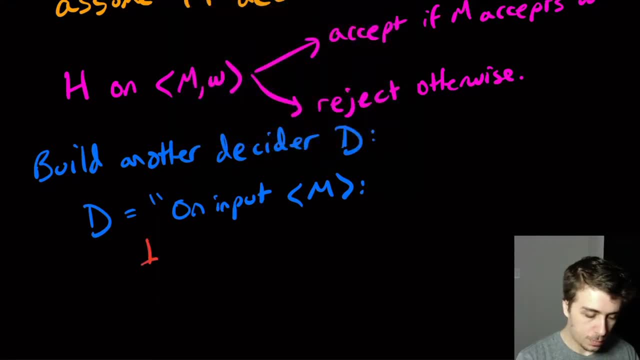 And what its first step is going to do is: it's going to run that supposed decider H upstairs. It's going to run H on, well, the H of the machine. So it's going to run H on the H of the machine. 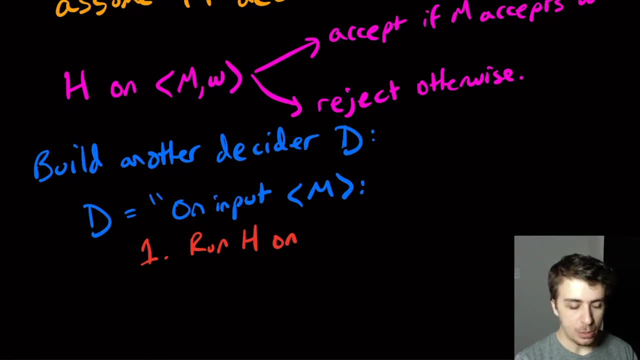 So it's going to run H on the H of the machine. So the H machine requires two inputs- right here You see, M and W- whereas the D machine only has one input: the machine. So we need a string as the input for the second parameter, for H. 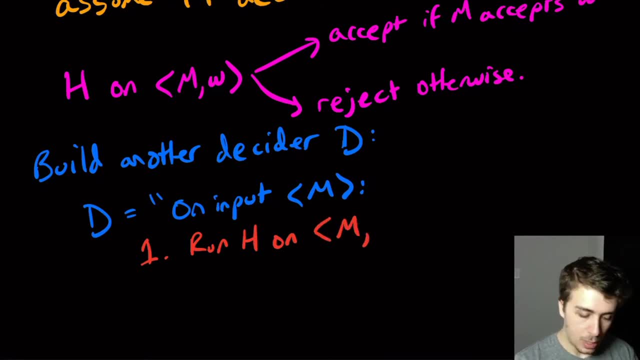 So I can feed M into the decider H here, but I need the input string. But one string that we can use is the actual string representing the machine itself. So remember that the angle brackets mean the string encoding of the thing. So here we're just feeding the string representing the machine into the machine itself, which is totally okay. 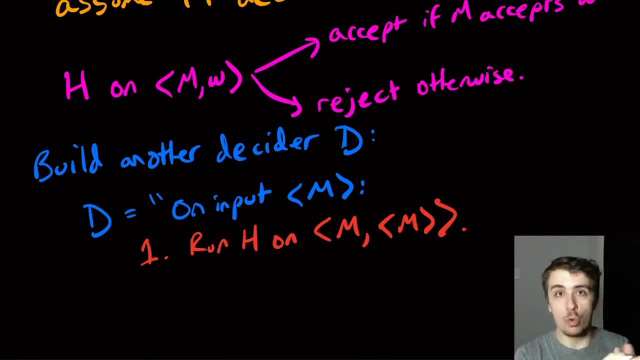 You could have a program send its own code as its input to itself. You can do that, And we're doing the exact same thing here. I'm not claiming that this machine has any purpose other than to derive a contradiction, Which is what it really is used for here. 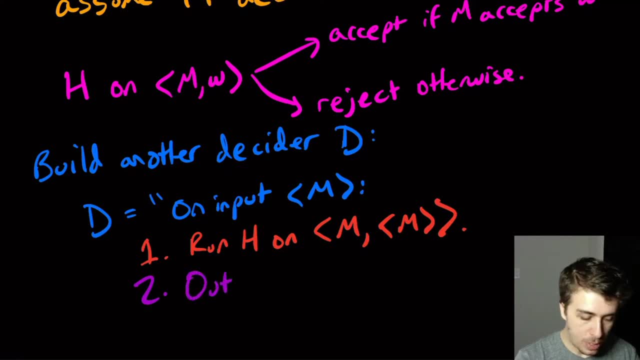 So the second step is output the opposite. So whatever the H machine says do the exact opposite of whatever it is. Well, this is a decider for whatever language. it is because the H machine runs in a finite amount of time, by assumption. 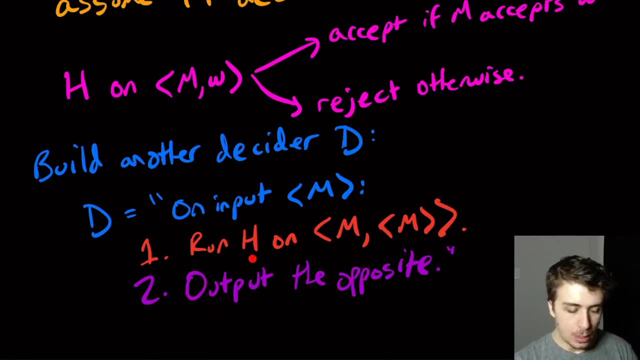 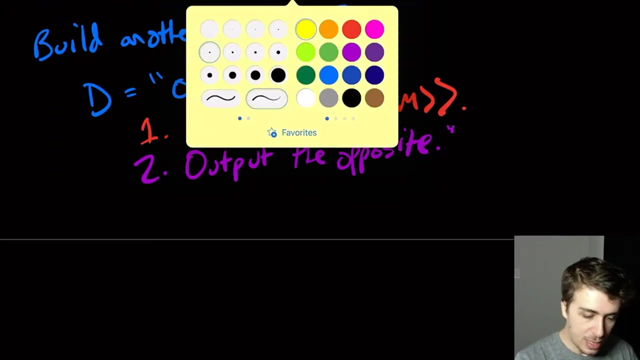 And clearly this runs in a finite amount of time. So if H says yes, we say no, Or if this thing says accept, we say reject. If H says reject, we say accept And it decides some language. So again for posterity we should figure out what the D machine does. 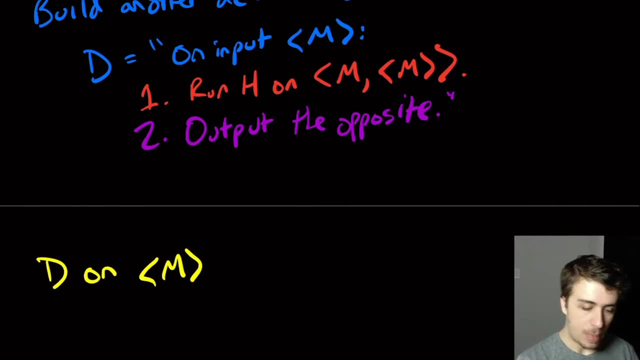 So D on the Turing machine M, remember it has exactly one input. It will always say accept or reject. Okay, We must do one of the two, because we argued that it was a decider. I didn't mean to underline that. 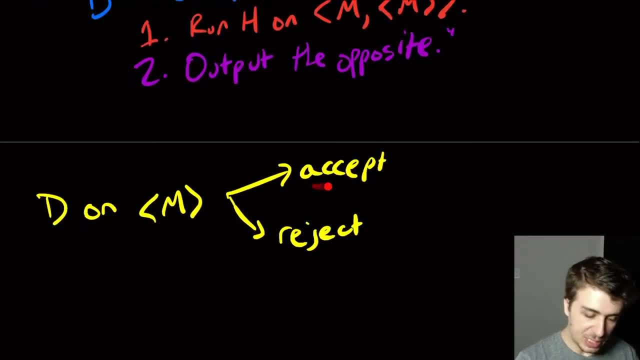 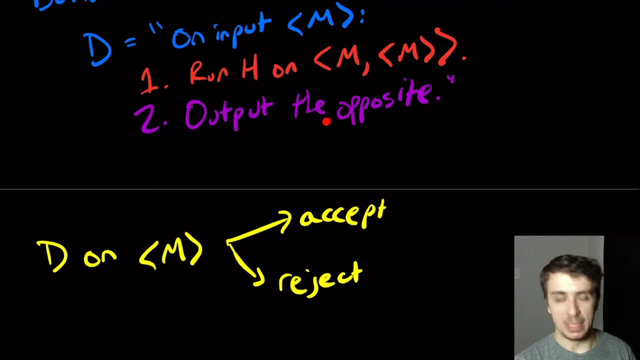 It runs in a finite amount of time, though, So it says: accept, if, what? Well, what does it mean for the D machine to say accept? Well, we outputted the opposite. So that means that the H machine must have rejected at that point. 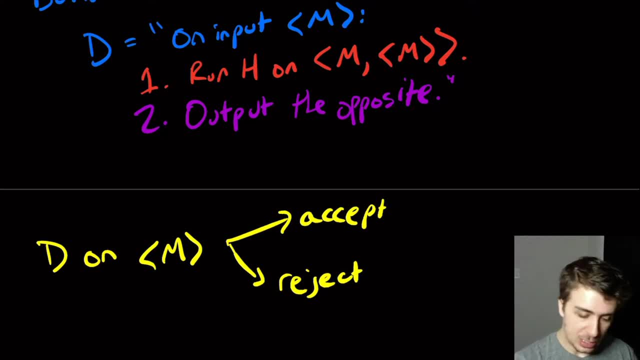 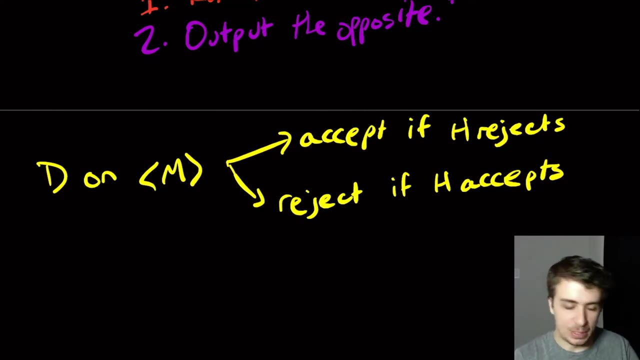 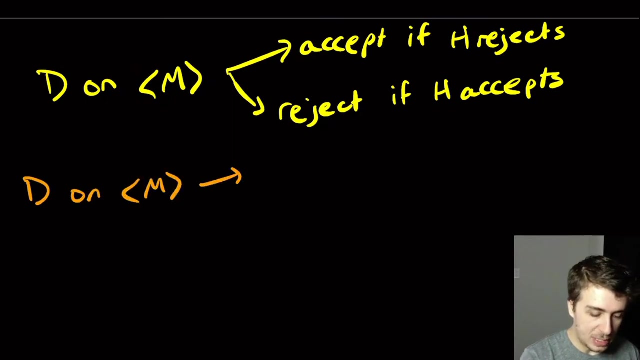 Because the D machine does the exact opposite. So this says: accept if H rejects And reject if H accepts. Okay, So it's just doing the opposite. So what I'm going to do here is I'm going to actually rewrite this in a different way. 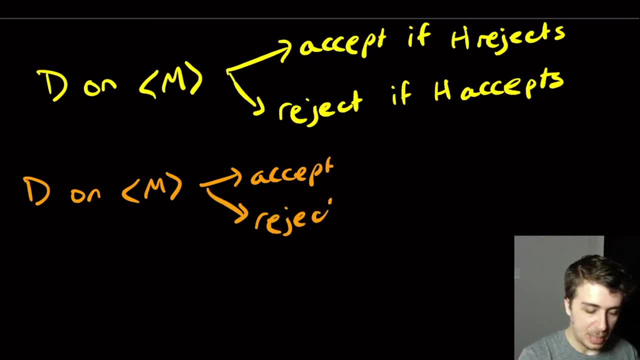 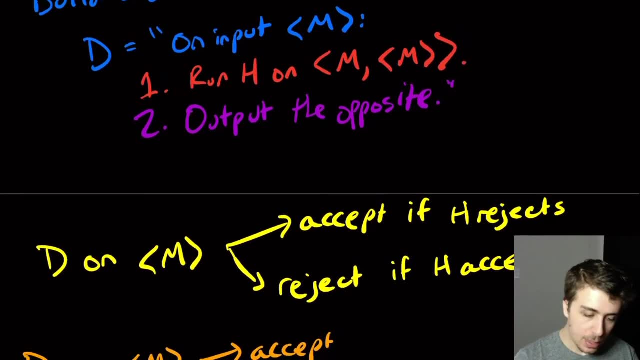 It's going to say accept or reject, So this part's exactly the same. But I'm going to expand on what H rejects means. So remember: H says I solved the ATM problem, which means that I figured out whether this machine- the first parameter. 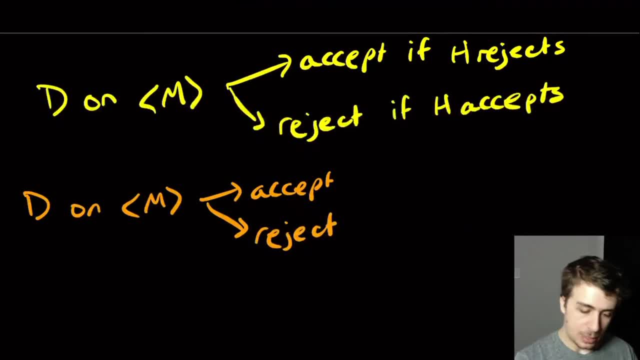 accepts the second one or not, And so this says accept if H rejects, Well, that means that the machine itself here, if M, does not accept its own string. So that's just what the H machine is. So the D machine says accept if the M machine does not accept. 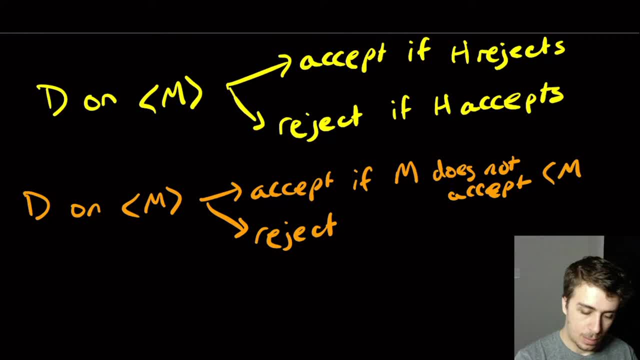 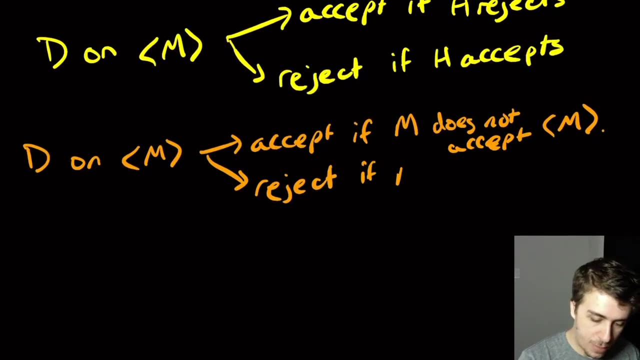 Accept its own string as its input, And that's totally okay. There's nothing inherently wrong with that. A machine doesn't have to accept its own string And it says: reject if M accepts its own string. Yeah, its own string, Okay. 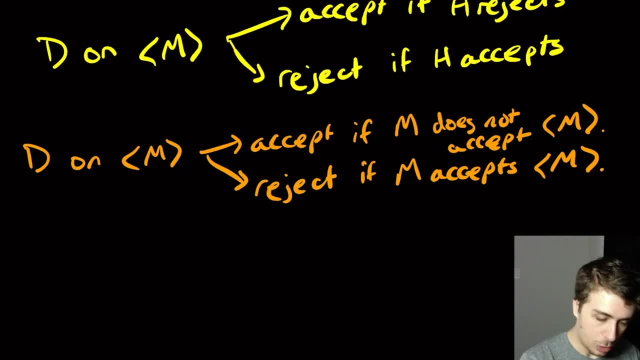 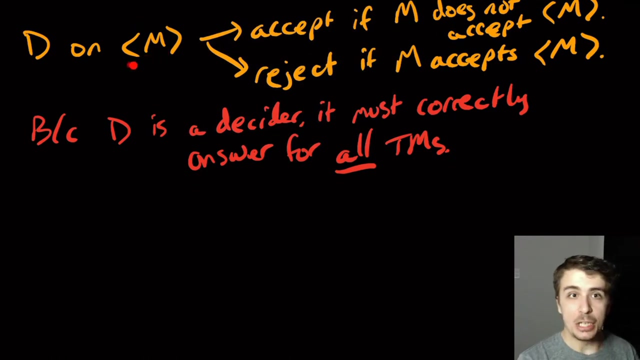 So because D is a decider- actually I'll even write this out- Because D is a decider, it must correctly answer for all Turing machines, right? Because it's a decider, including itself. So if we instead say: well, what if we feed D's own string, the machine D? 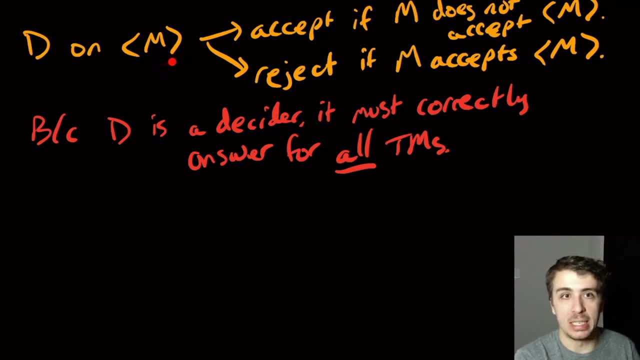 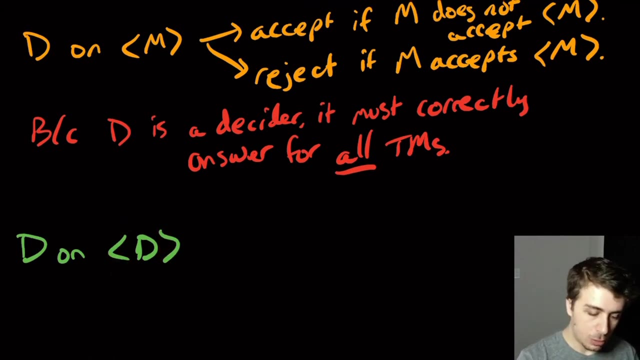 to itself, Because I can feed any Turing machine into here And D is a Turing machine And we can certainly do that. So let's see what happens if we try to run D on its own source code in some sense. So it's going to again say accept or reject. 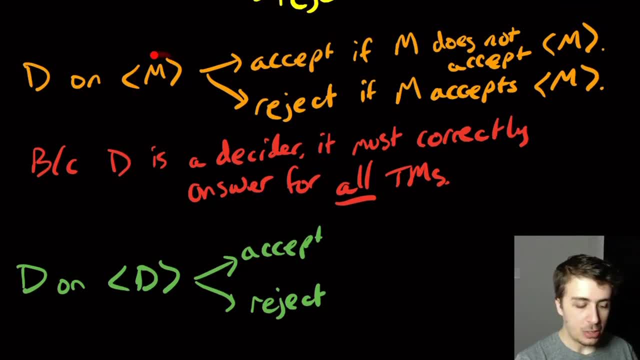 And what you can actually notice is the only thing that changed here is the M part. So everywhere we see The M over here. I'm just going to replace it with D. So this says accept. if D does not accept, D Wait. 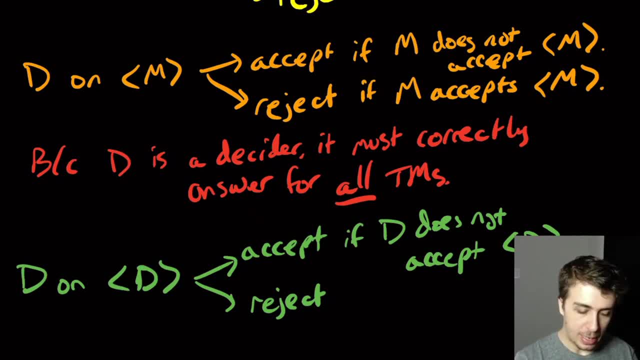 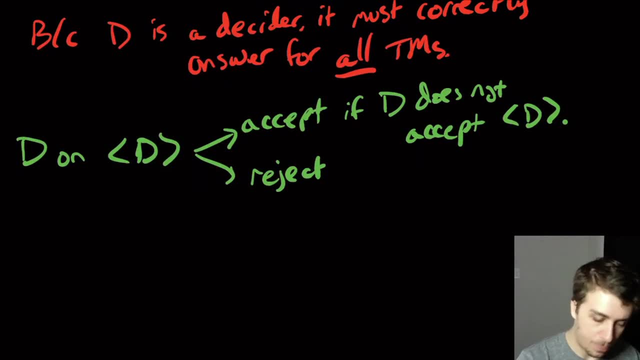 So D accepts its own string. if D does not accept its own string, That makes no sense. Okay, Well, let's try the other one: Reject. if D accepts, Rejects D. Wait. So D rejects its own, encoding its own string, the code representing it. 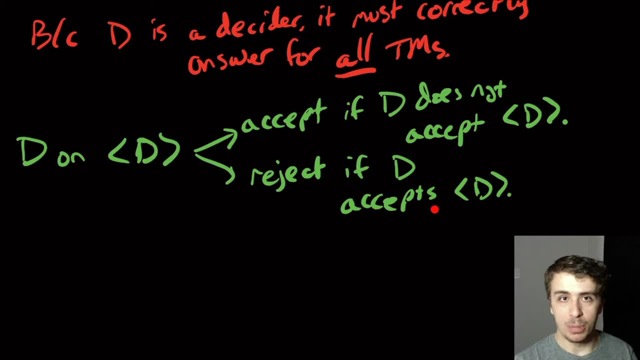 If it accepts it. Wait, that's impossible. So that's the contradiction. So this means that D cannot exist. This machine cannot possibly exist because we assumed that it was a decider, which means it must correctly get the right answer On all inputs, but it just got it wrong on at least one input. 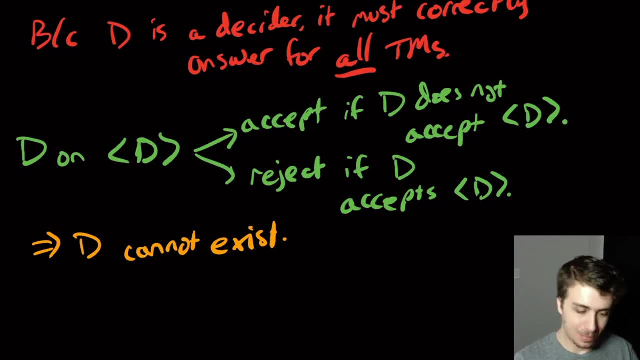 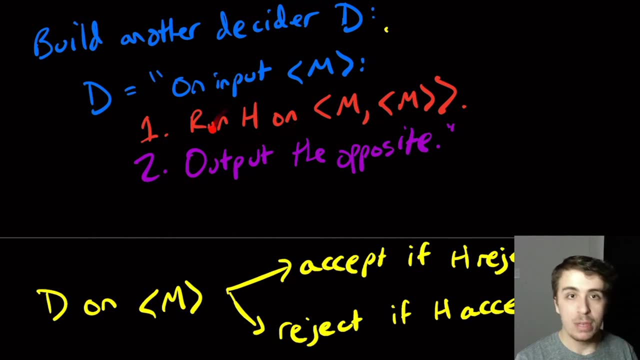 So, therefore, it's not a decider, and so it cannot exist. The only way that this could happen, though, is the only thing that we really relied upon to build this machine D was the construction of this H machine, So there's no other assumptions here other than this one.